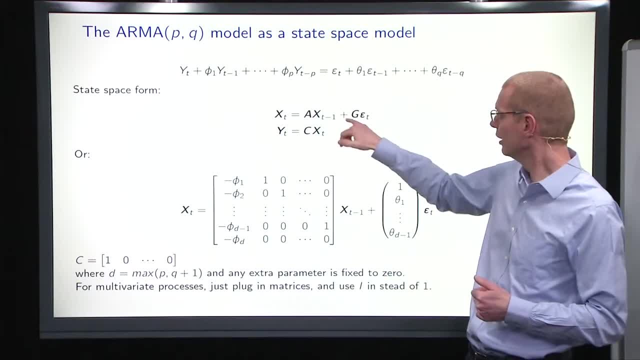 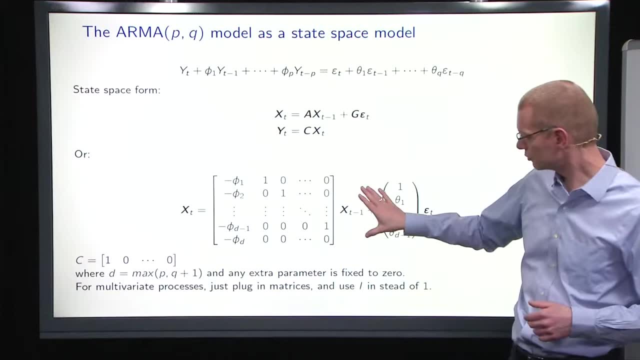 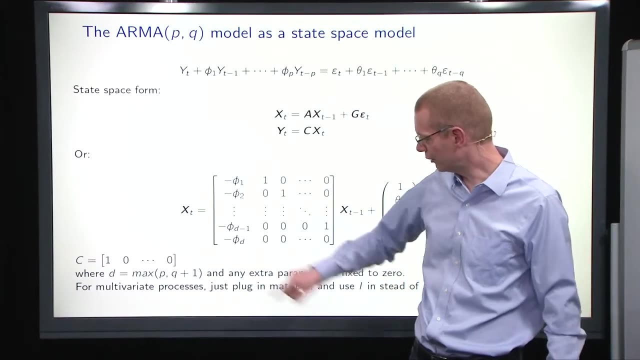 add that later if needed in particular case. And then the noise up here is only univariate, Whereas in the general setting it's multivariate. So what we do is that we take all the AR coefficients here parameters put that in the first column with negative sign, and then we put a unity matrix here. 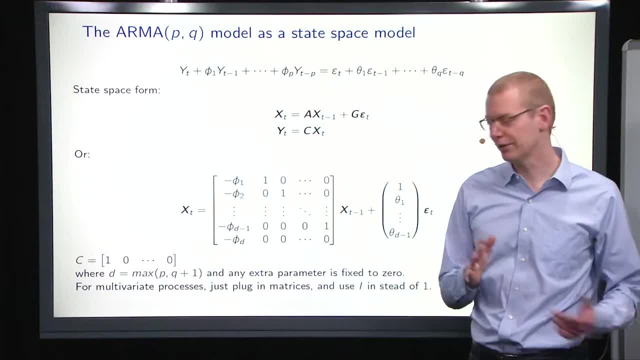 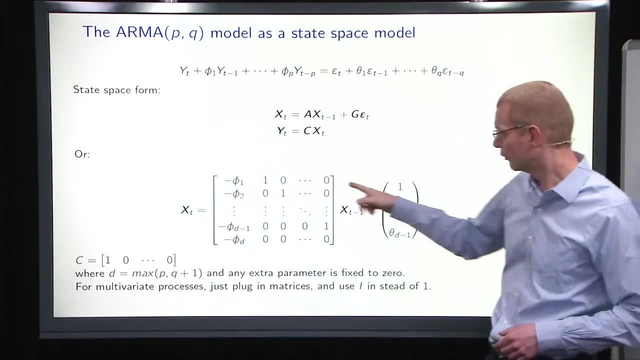 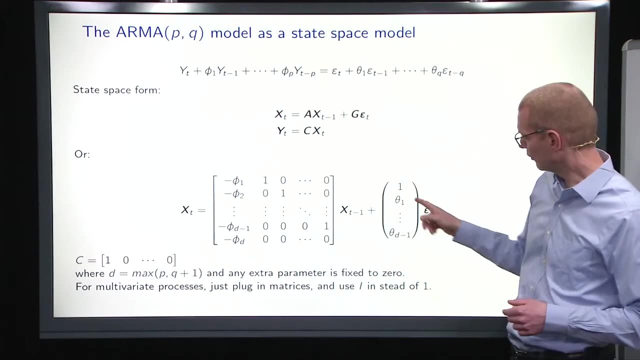 and end out with a row of zeros in the bottom. That's the general setting. Then we have, for the moving average part, We have start with a one because we want the first element of the x state here to represent time t and then which we have to have epsilon t there and then we can take if there are moving. 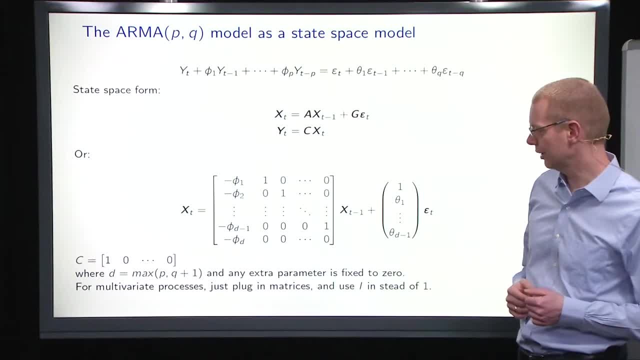 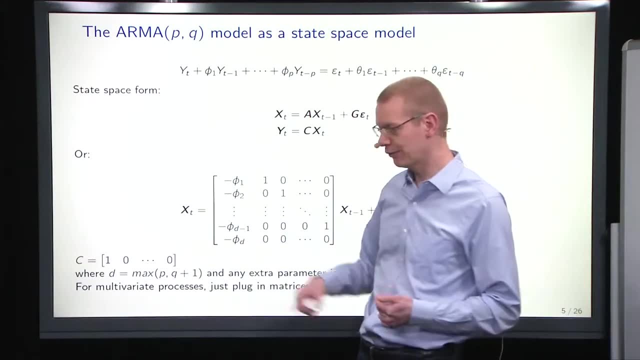 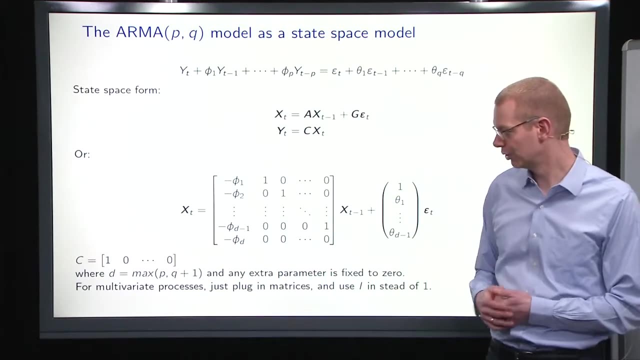 average parts. we add those up into the equation there. Now, of course, you may not always have as many thetas and phi's as in this particular case. So we have d there and d minus one there, and some of these may be zero. So the order of the dimension of this is either: is the maximum of p? 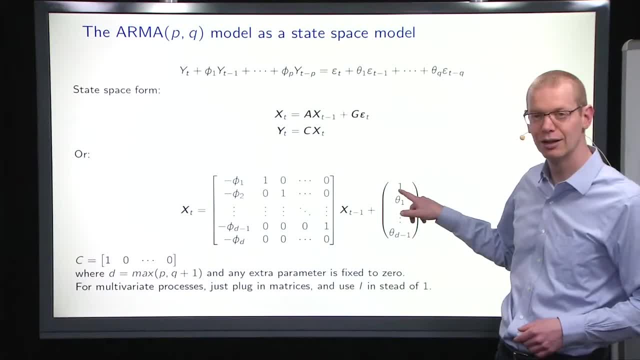 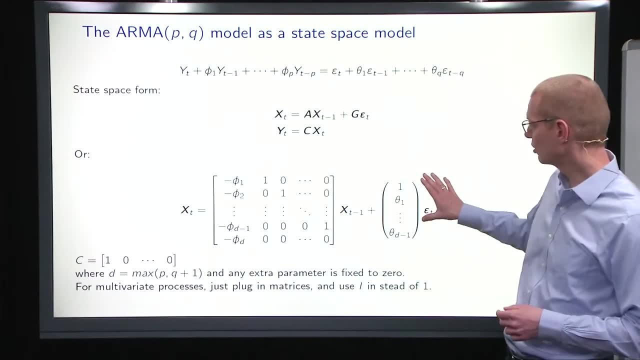 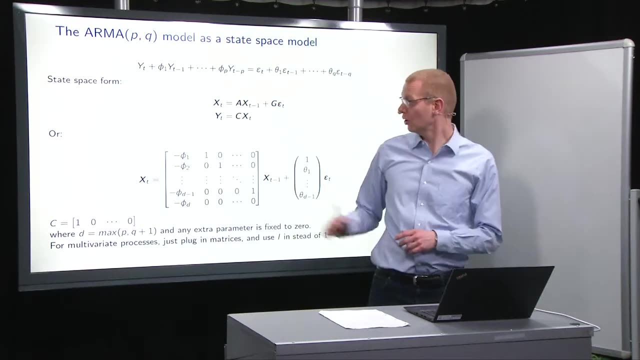 and q plus one. The q plus one comes from the fact that you need this one up here to keep track of that. So how does this work in practice? Let's just look at a simple model and see can we actually understand what is going on? So let's make an example of an AR2 model. 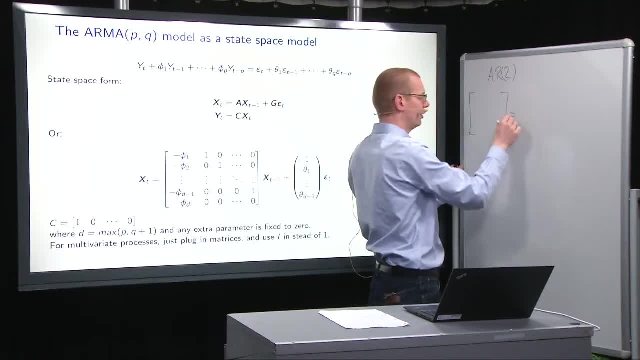 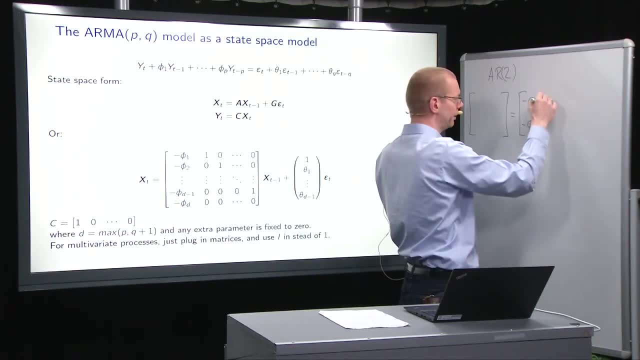 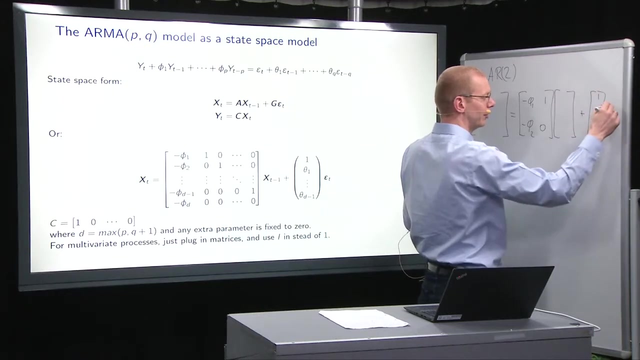 We're going to look at what the process comes out. We're trying to fill in the gaps. Let's fill in first what is known. We have the system matrix here with a unity matrix of dimension one, and then a row of zeros, and then what was the state before? and then epsilon is a one zero on epsilon t. So 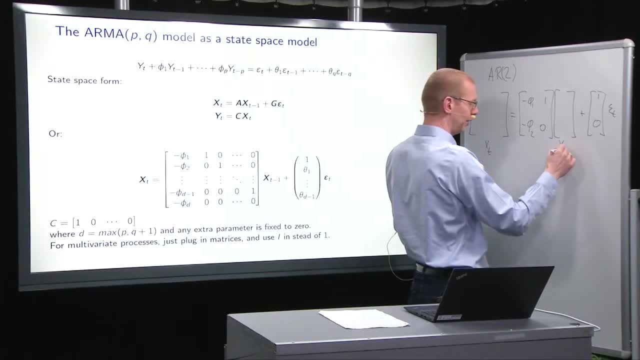 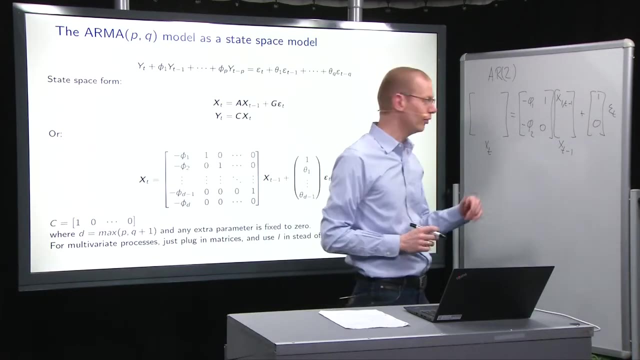 what we have over here is we have x, t minus one, and if we just fill in an element, what we have up here at the first element is x, one comma the time, t minus one. So given this number up here, we can see what are we going to get. 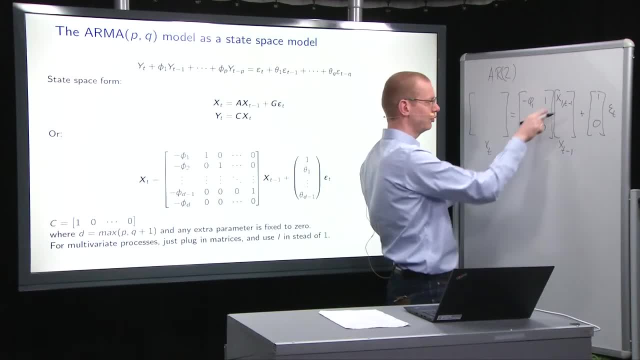 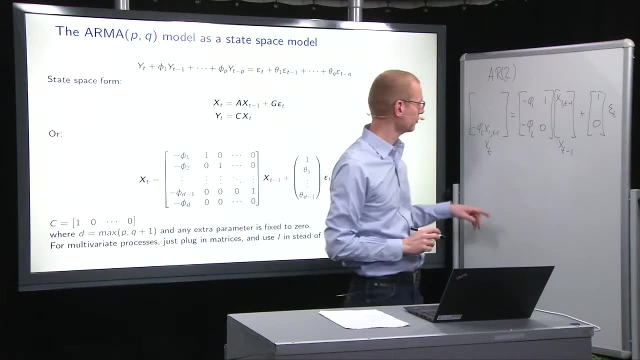 in the second element at time t, We're going to get minus phi two of this one up here, So minus phi two x one comma, t minus one. Now, given that we have this, then when we then look forward once a forward in time, this will: